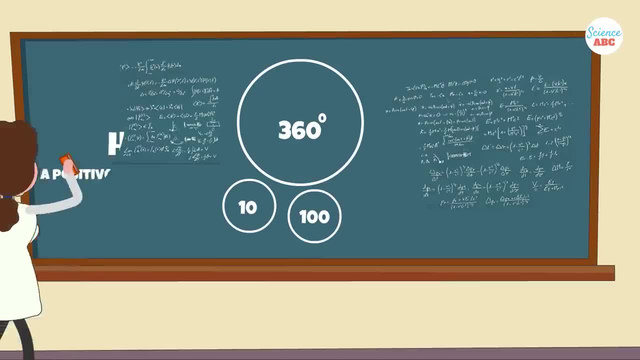 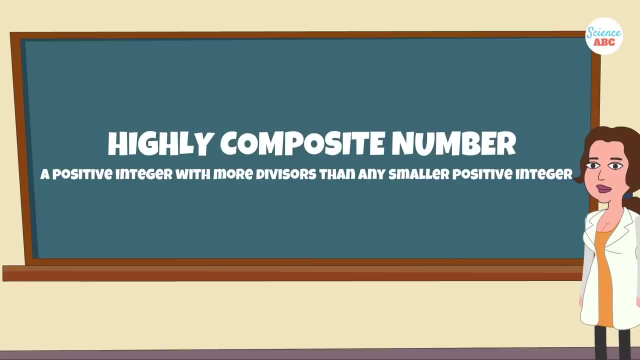 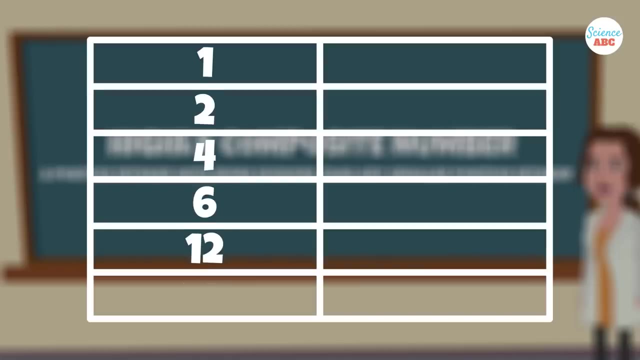 such as 100, has only 9 divisors. Numbers are said to be highly composite if they are positive integers with more divisors than any smaller positive integer has. The only highly composite numbers below 360 are 1,, 2,, 4,, 6,, 12,, 24,, 36,, 48,, 60,, 120,, 180, and 240.. Highly composite numbers. 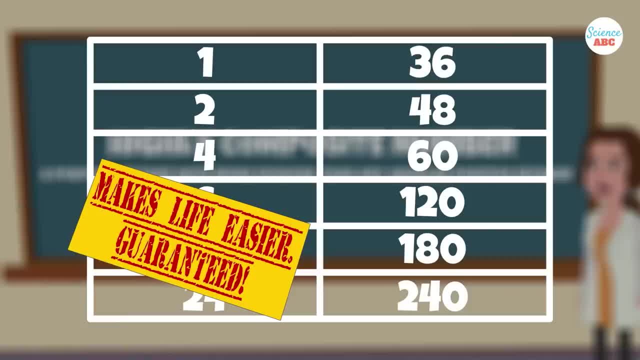 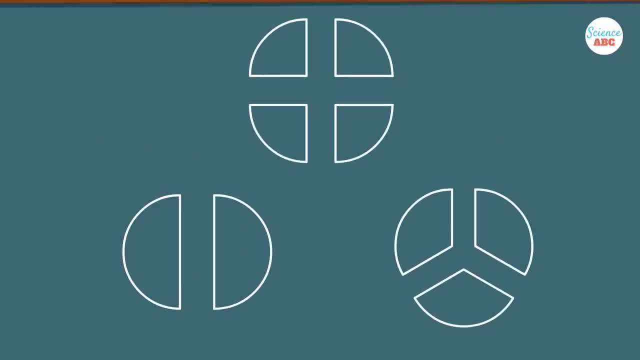 are considered to be highly composite if they are positive integers with more divisors than any smaller positive integer considered good base numbers with which to perform common calculations. For example, 360 can be divided into 2,, 3, and 4 parts, and the resulting number is a. 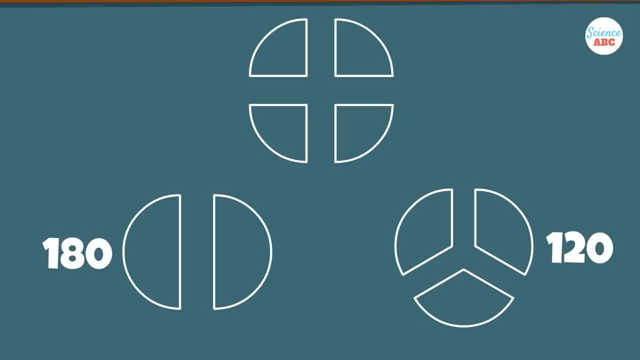 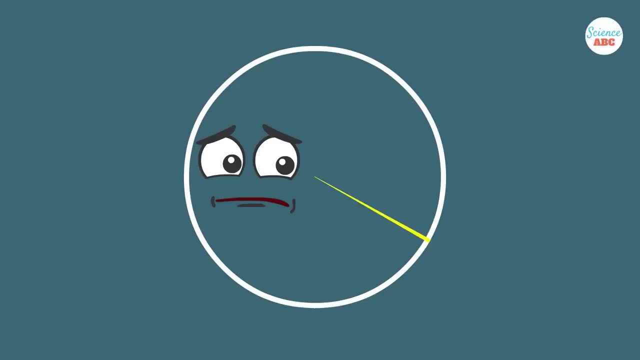 whole number. The resulting numbers are 180,, 120, and 90.. However, dividing 100 by 3 doesn't end in a whole number. Instead, it provides a decimal value of 33.3, recurring, which makes performing calculations. 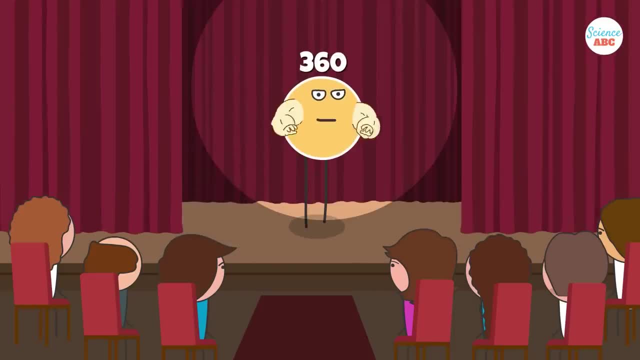 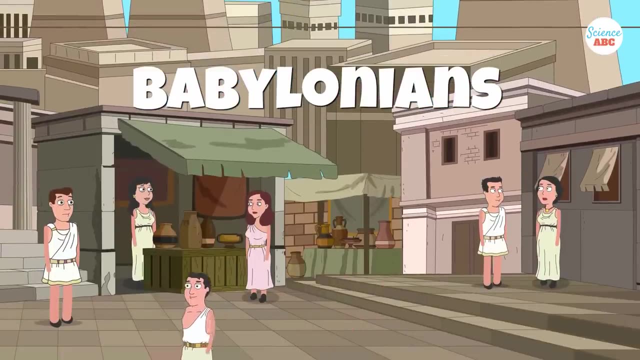 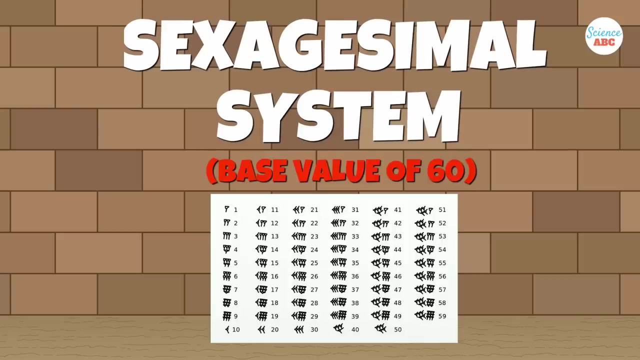 much more difficult. Systems using 360 are quite simple once you become used to them. One theory for why a full circle is 360 degrees comes from the Babylonians. The Sumerians and Babylonians used the sexagesimal numeral system, a system with a base value. 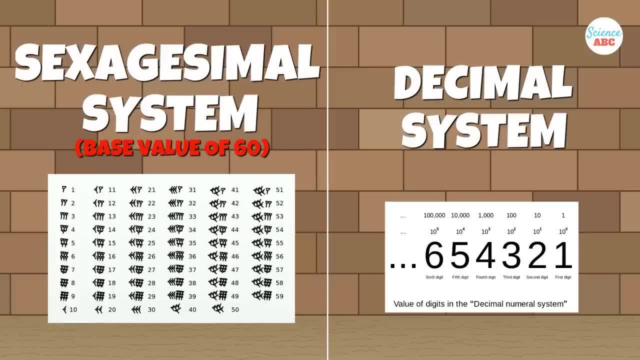 of 60,, while the current system we use is known as the decimal system and has a base value of 10.. So once we reach the 10th number, we start repeating the symbols or previous numbers from 0 to 9, to form new numbers. 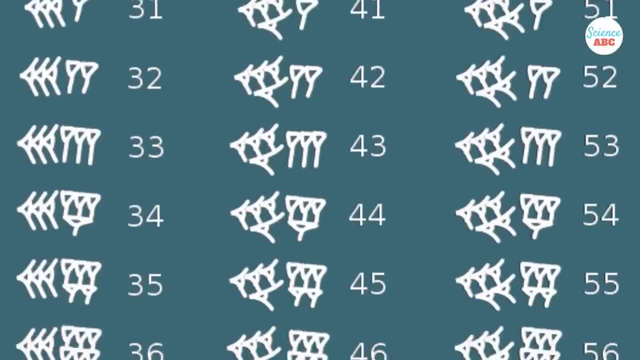 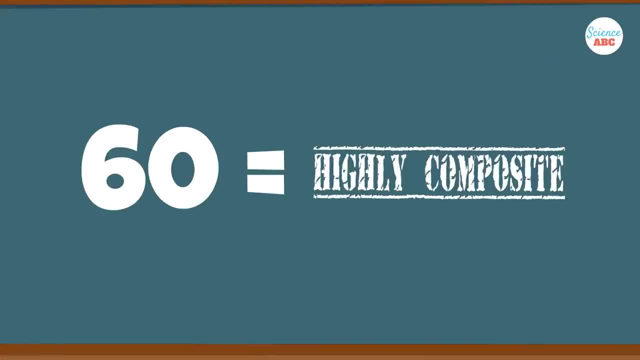 The Babylonians used the hexadecimal numeral system to form new numbers. The Babylonians had 60 different symbols with which they formed numbers. Again, why would they use 60? Because 60, just like 360, is a highly composite number with up to 12 factors. 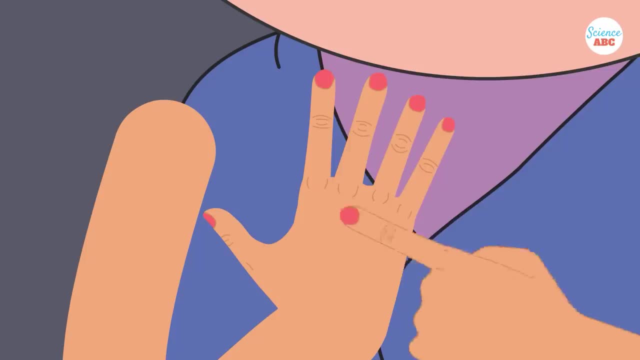 Just as we can count 10 on our fingers for the decimal system, we can also count to 60. Start by counting the knuckles of the 4 fingers, not the thumb on your right hand: 12, right Now, on the other hand, raise any of those fingers to note that you finished one iteration. 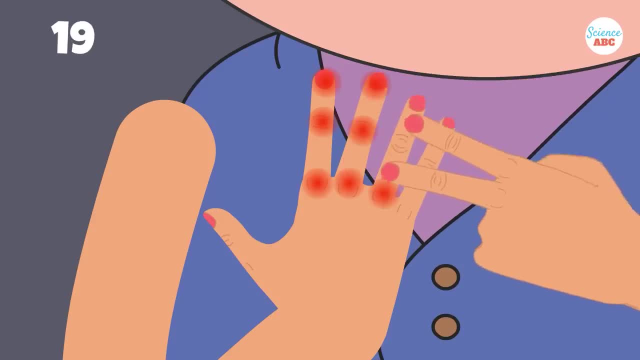 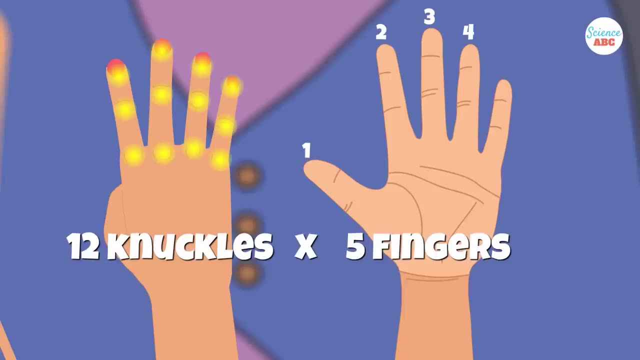 and got the number 12.. Now repeat the same procedure as many times as the number of fingers remaining on the left hand. The number you will end up with is 12 knuckles times 5 fingers, which equals 60. Now to tie this all together, if we were to draw an equilateral triangle with the length,